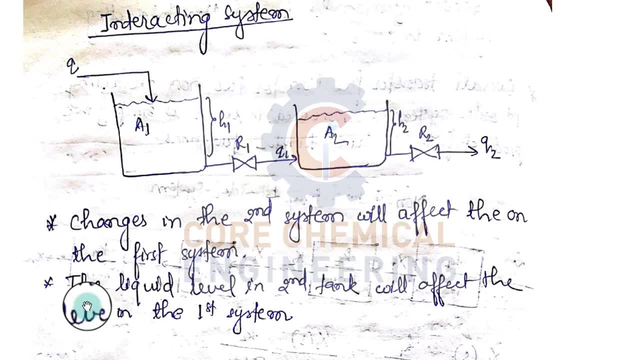 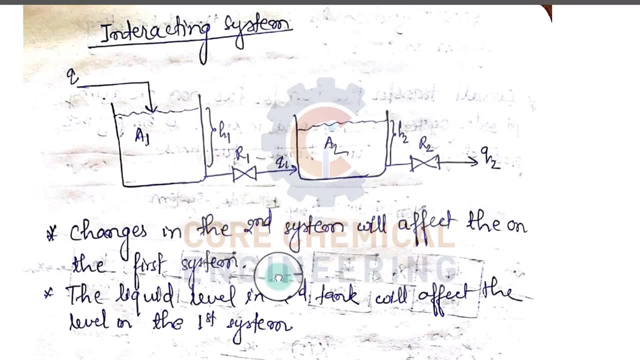 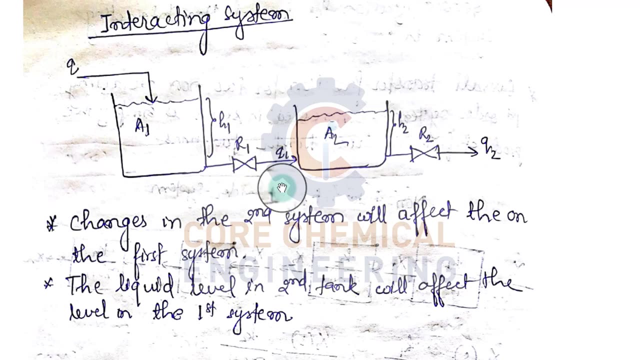 effect on the first system, and then liquid level in the second time will affect the level in the first time. that's what I told you. now let's do the mass balance. so what we need to find out? first of all, we'll try to find out h2s divided by Q. office for this. 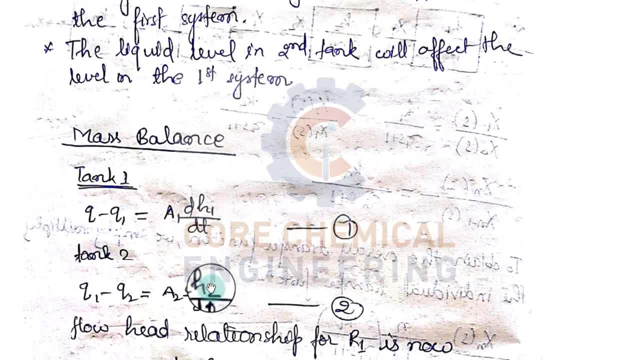 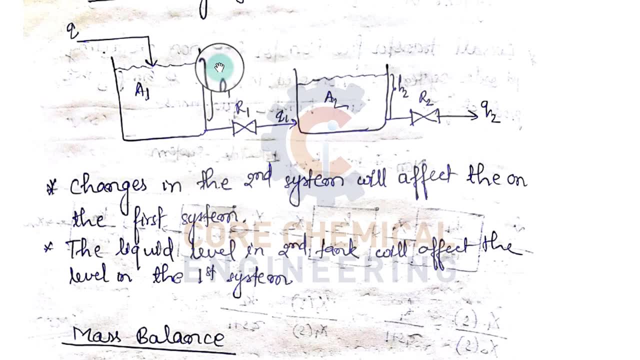 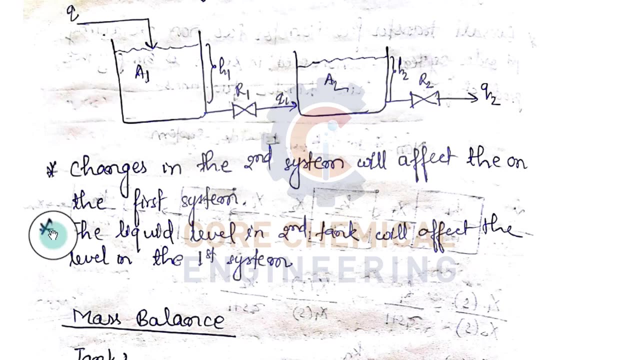 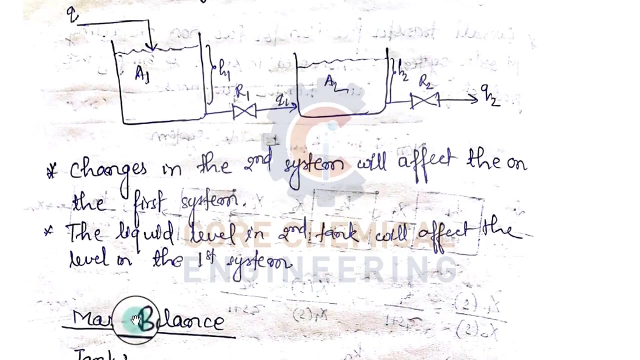 interacting system. so let's do the mass balance, okay. so if you want to do the mass balance, so Q minus Q n equal to even into DH, 1 by DT. okay, so for the first time will do so. Q is your fluid, okay, and here density is constant. basically, if you want to do the mass balance, then in that case you have to multiply flow rate with the density, but density will be common in all, so it gets eliminated. that's why I have not written it here so directly. I have written here with respect to the flow rate, right. so q minus qy is equal to a1 into dh1 by dt. 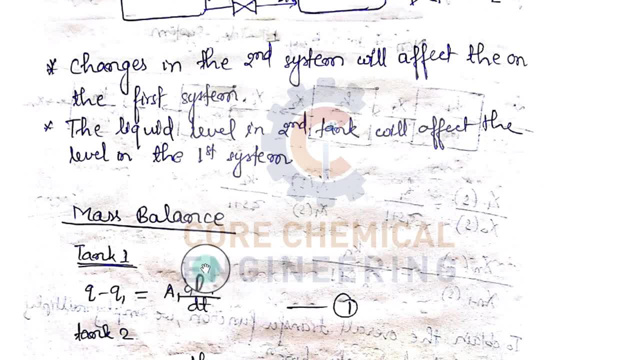 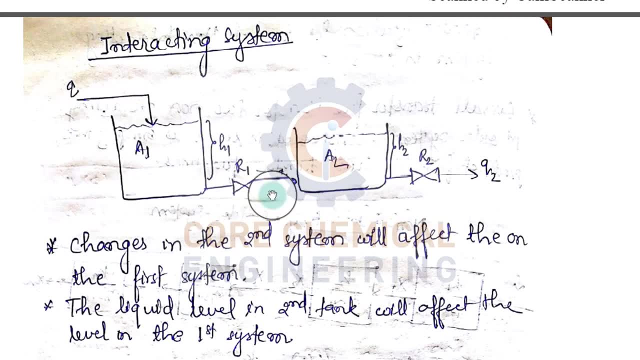 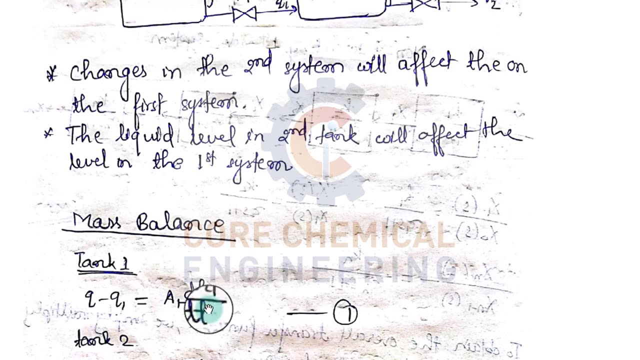 a1 into h1 is your volume, and if you like a differential with respect to time, okay, then it will. it will comes flow rate right. so q is inlet, q1 is your outlet. in minus out there is no generation or anything added externally. in that case is equal to a1, dh1 by dt. 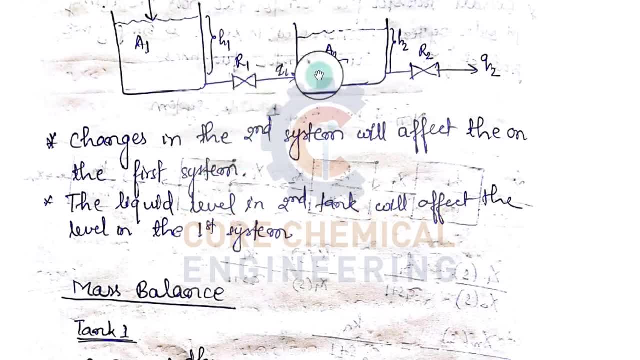 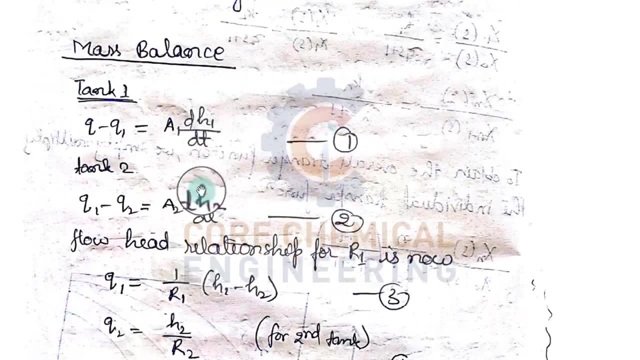 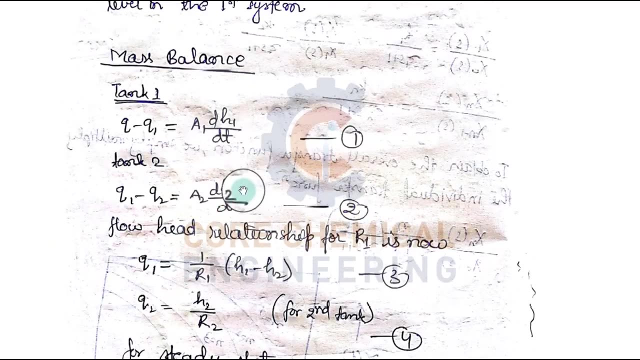 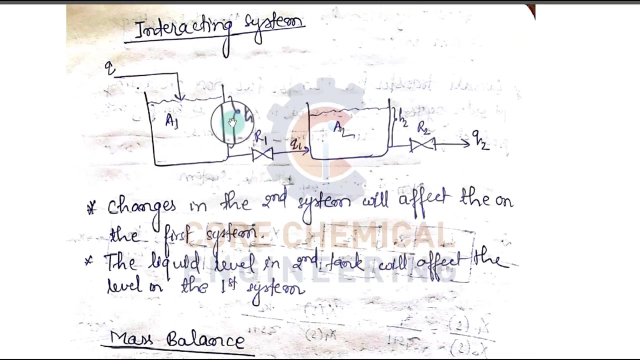 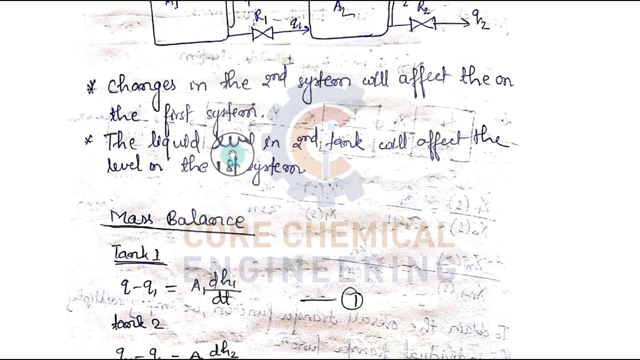 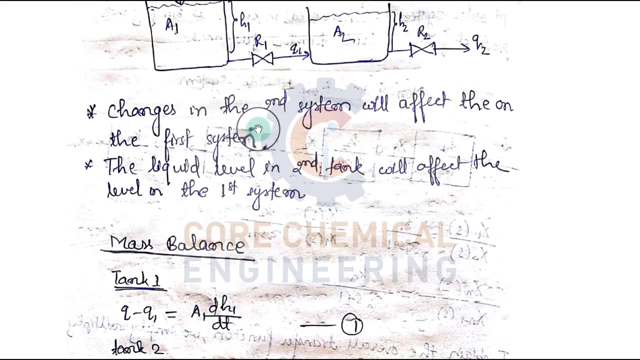 similarly for tank 2 inlet is your q1. q1 minus q2 is equal to a2 into dh2 by dt right. a2 is the cross section area for the tank 2. now follow head relationship for r1 is now: now, if you want to do r1, is your flow resistance, for that your q1 would be what will be your q1 flow rate? your q1 flow rate will be now h1, your height, h1, minus of your height, h2, because you are getting this much height head only for the flow, because it has already leveled in that. so for that q1 qn is equal to h1 minus h2 by r1, whereas q2 is equal to h2 by dh1 by dt. 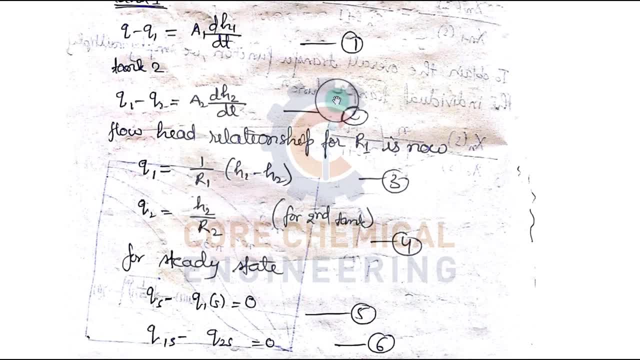 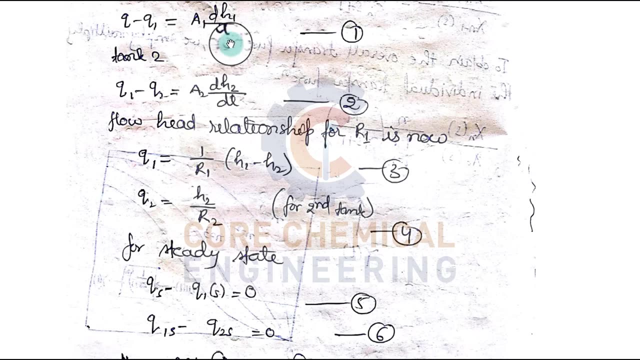 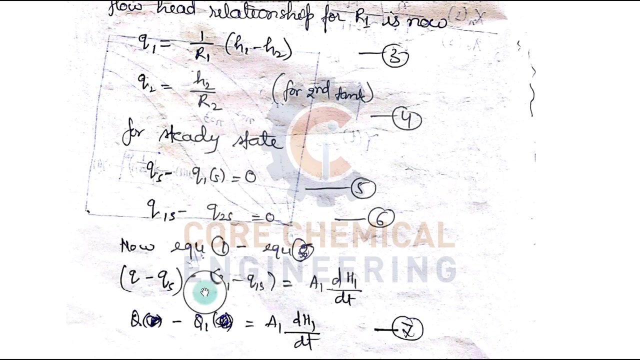 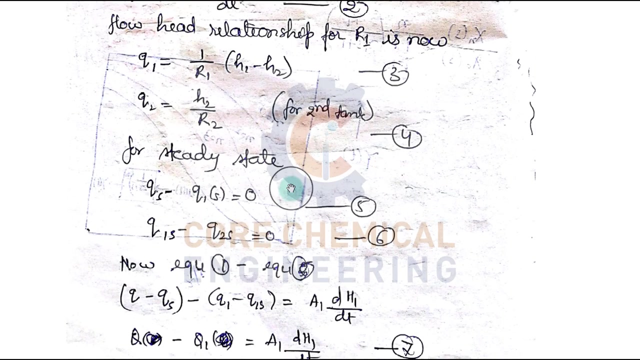 right, so q1 is equal to h2 by dh1 by dt, right? ok, now you have to subtract equation 1 minus. this is for normal and this is for this is for a steady state. so we have to do equation 1 minus. equation 5 will get Q. 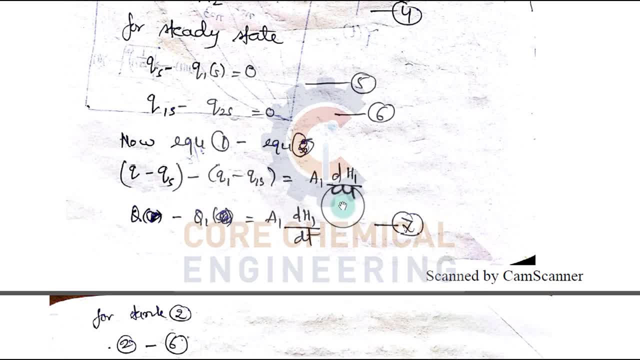 minus Q s minus Q 1 minus Q s, equal to a1 dh1 by dt right. so overall this value will will get. this is the deviation form. this is Q minus Q 1, minus curious is you. Q 1 minus Q 1 s is equal to Q. 1 is equal. this is the Q 1 is your. 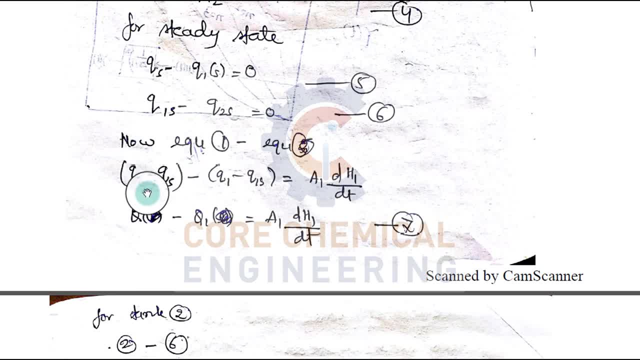 deviation form of this value and Q is the deviation form of this value. Q minus Q s steady state value. this is the current deviation form. Q minus Q 1 is equal to a1 into dh1 by dt right. similarly for time 2 we can write: okay. 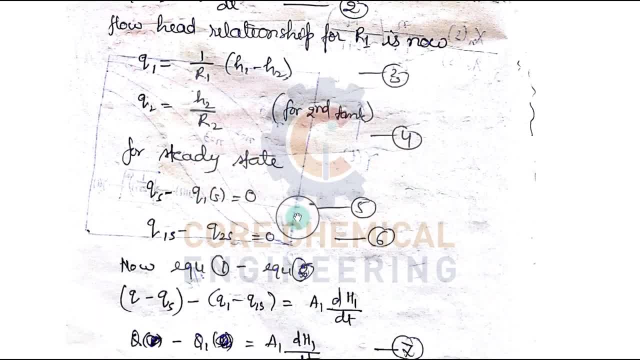 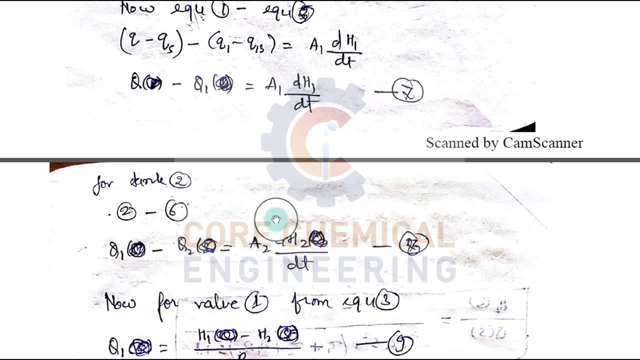 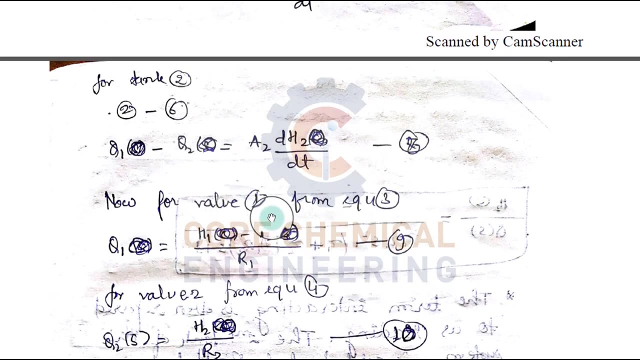 for time 2. if you want to write, you have to do equation 2 minus equation 6. so let's do. we'll get this value. Q 1 minus Q 2 is equal to a2, dh2 by dt, right by duty. now from equation one. now for the value of one from equation three. so 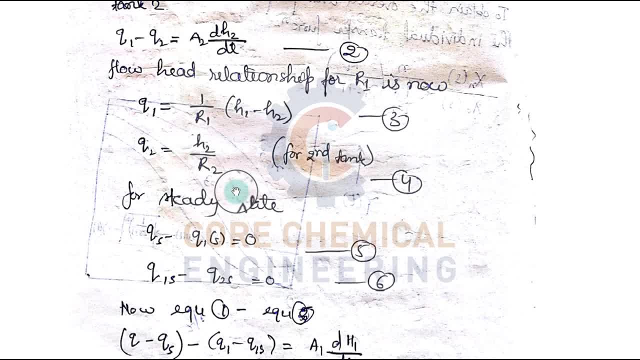 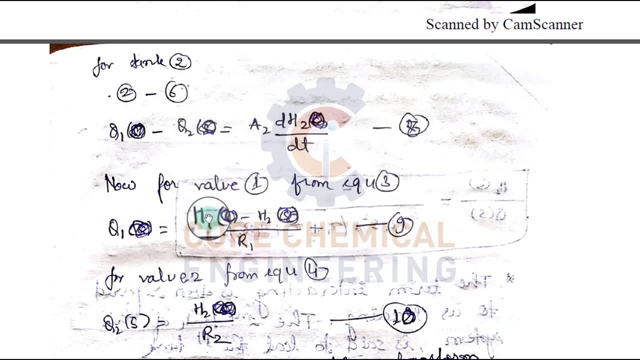 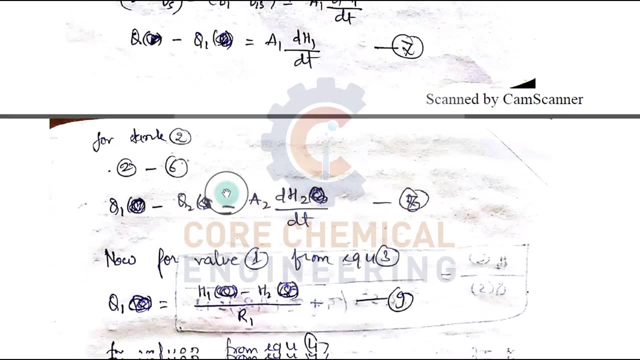 we have to see. this is the equation three. so it's mega occurs. the time loop is Kabila plus transform later. so let's take the left last term from this also, it will becomes: Q 1 is equal to h1. Q 1 is equal to h1 minus h2 divided by r1. for 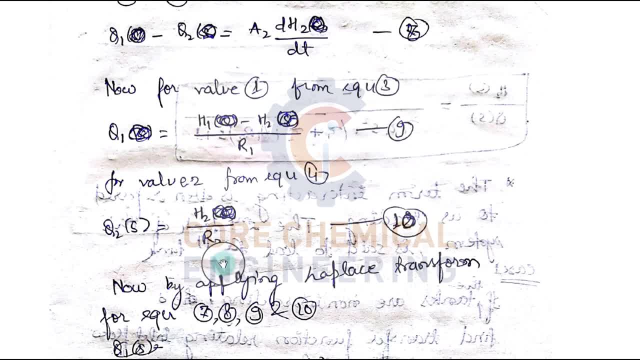 wall to. similarly, we can add: as Q is equal to h to the r1, Q 2 is d, or by h, Q 2, h to the r2. right now, what we can do now, we can apply the localization, we can apply the localization, we can apply the localization. 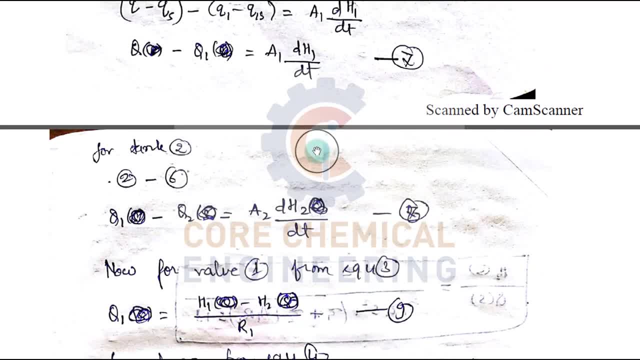 Laplace transform for equation 7,, 8,, 9,, 10.. So we have to apply the Laplace transform for equation 7.. Similarly for equation 8.. Similarly for equation 9.. Similarly for equation 10.. 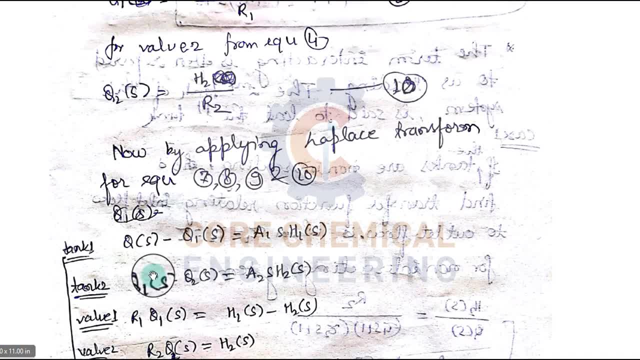 We will get here the four equations. right, These are the four equations. For tank 1, we will get Qs minus Qn is equal to A1 into S, into H1 of S. Similarly, for tank 2, we will get this value. 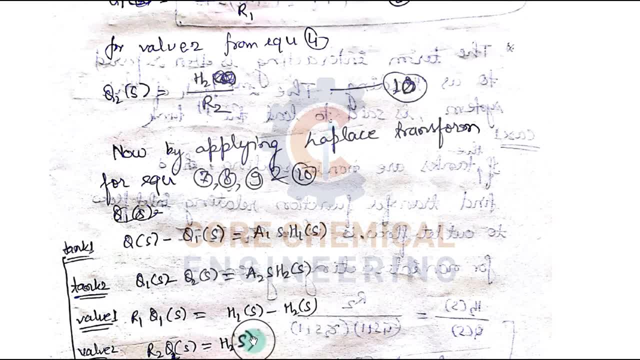 For valve 1, we will get this value And valve 2, we will get this value. So we have basically how many constants we have gotten: 1,, 2,, 3,, 4, 5.. 5 unknowns and have 4 solutions. 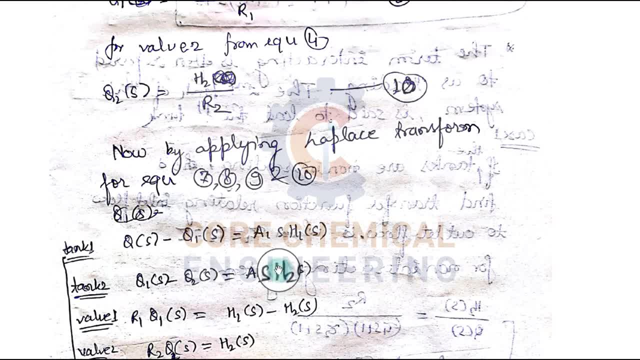 So what we can do, We can get the value of H2S divided by Q of S by eliminating H1, okay, H1S and Q2S- okay, And QnS- right. So we eliminate all these three. 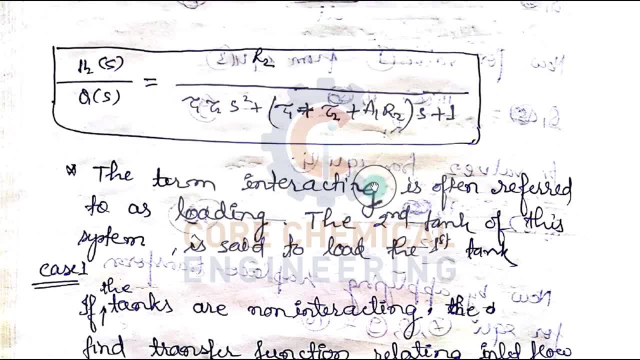 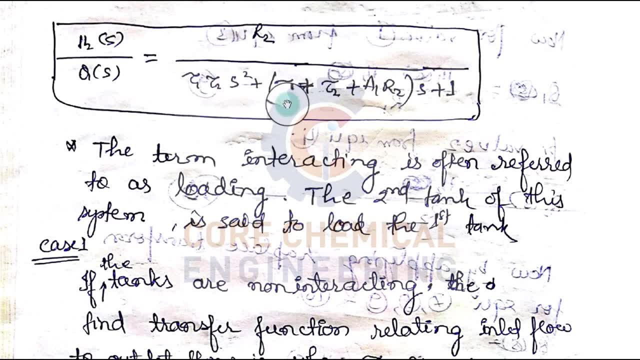 By solving these equations we will get finally this equation: H2S divided by Q of S is equal to R2 divided by tau 1 into tau 2, S square plus in bracket tau 1 plus tau 2 plus A1, into R2 in bracket S plus 1.. 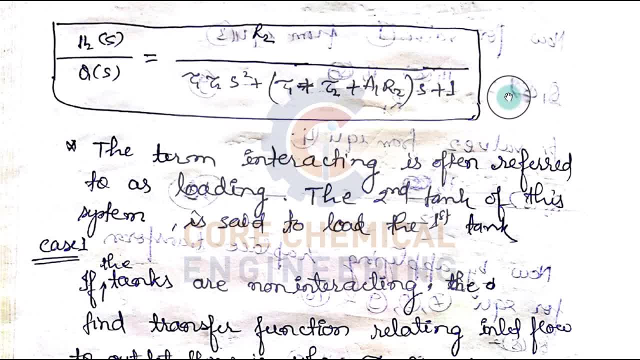 So this is very, very important okay, formula that you must remember before you are going to enter into any competitive exam, Like a GATE exam. if you are going to write for GATE exam, you must remember, Remember this formula, okay. 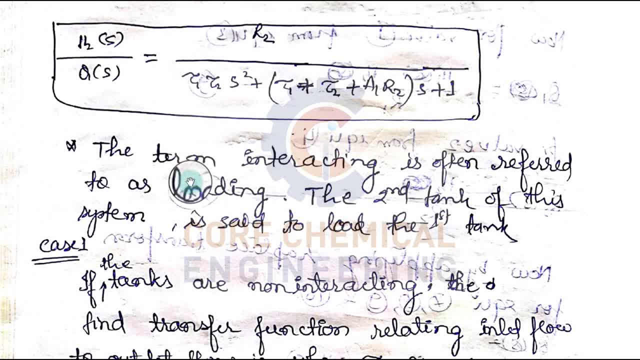 This is for non-interacting system, So the term this is for interacting. sorry, This is for interacting system, So the term interacting is often referred to as loading. okay, The second tank of this system is said to be the load to the first tank. 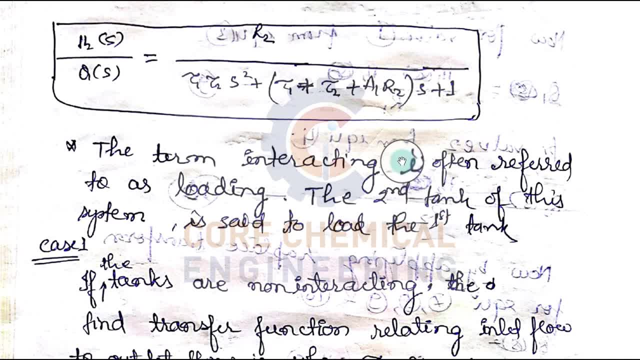 because it has already leveled. If you want to flow, have a flow from the tank 1 to tank 2, then if there is already leveled in the tank 2, that level will cause a resistance to the resistance to flow for the first time. 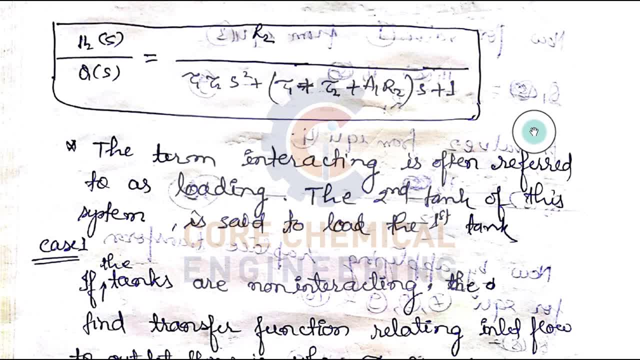 Okay, Okay, Okay, Okay, Okay. So in that term you can consider: as tank 2 is a loading, tank 2 is acting as a loading for with respect to the tank 1,. right Now, case 1, let's take the two cases. 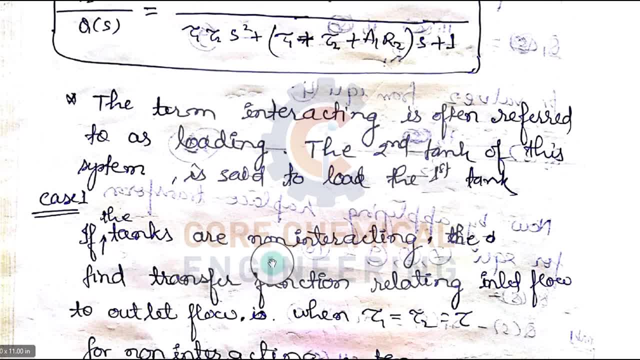 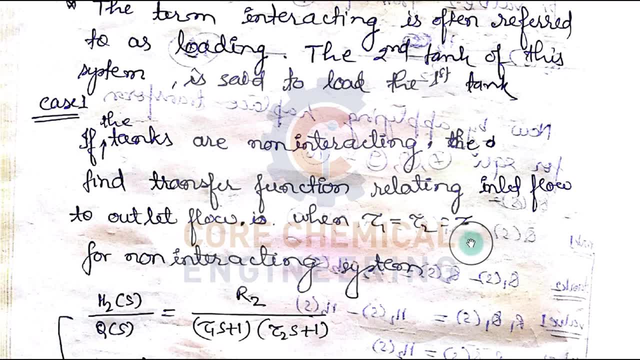 Case 1, if the tanks are non-interacting, and then in that case find transfer function relating to inlet flow rate to outlet flow rate when tau 1 is equal to tau 2 is equal to Q means you have to find Q2 divided by Qs right. 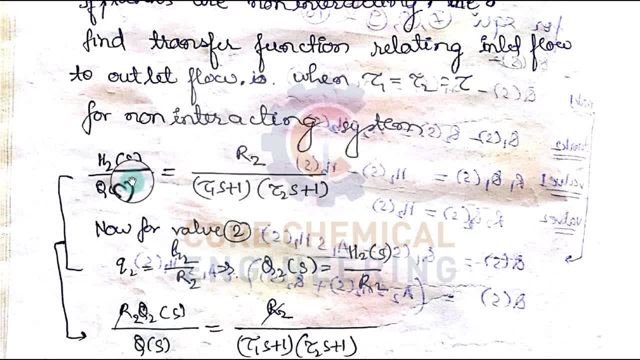 So in that condition what we will get For non-interacting, We know for non-interacting system: h2s divided by Qf is equal to r2 divided by tau 1s plus tau 1s plus 1 into tau 2s plus 1.. 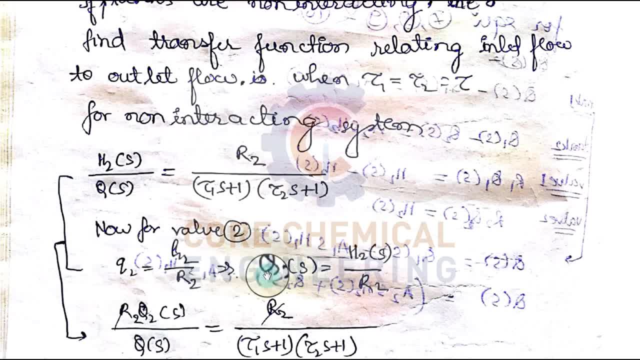 So we know that Q2 is equal to h2 by r2 is equal to Q2 of s is equal to h2s divided by r2.. So for that case we can put instead of h2s we can write as Q2s into r2.. 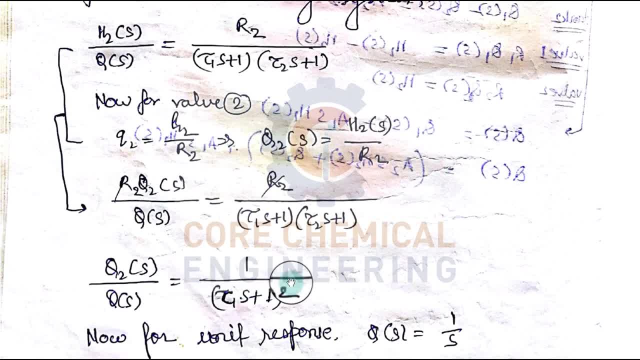 So if you put this, we will get: Q2s divided by Q of s is equal to 1 divided by tau 1s plus 1 whole square right, Because here tau 1 is equal to tau 2.. So one condition has been given. 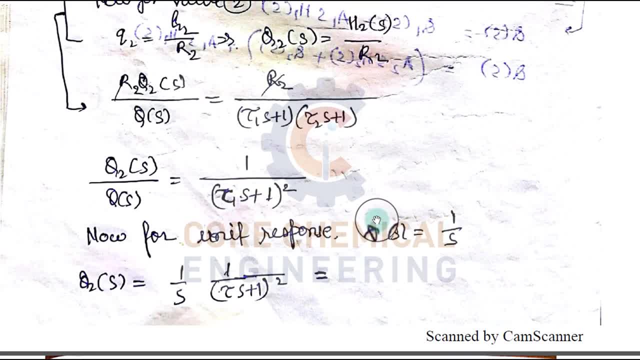 Now for the unit response. if you are going to put give input response, in that case Q of s is equal to 1 by s. So Q2 of s is equal to 1 by s into 1 divided by tau s plus 1 whole square. 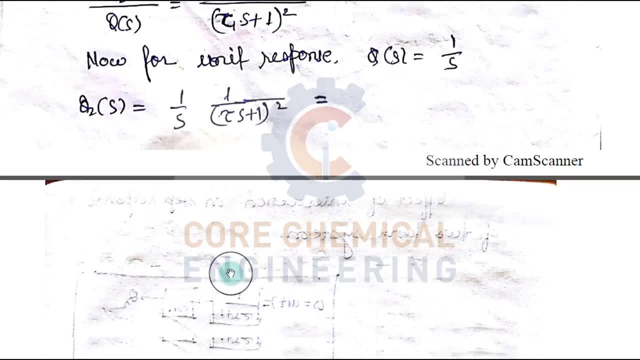 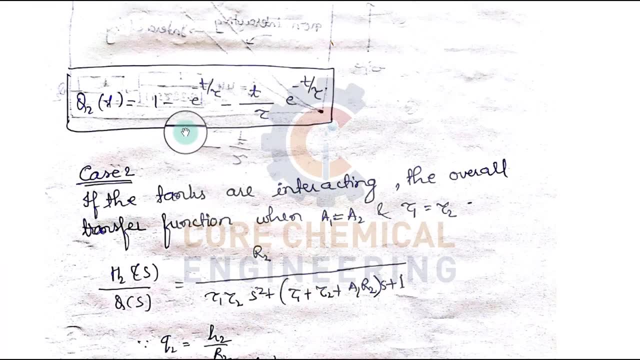 Now if we do the Laplace transform of the taking inverse Laplace transform of this equation, okay, you solve it mathematically somewhere. practice it, you will get. Q2 of t is equal to 1 minus e, raised to power minus t by tau, minus t by tau, into e raised to power minus t by tau. 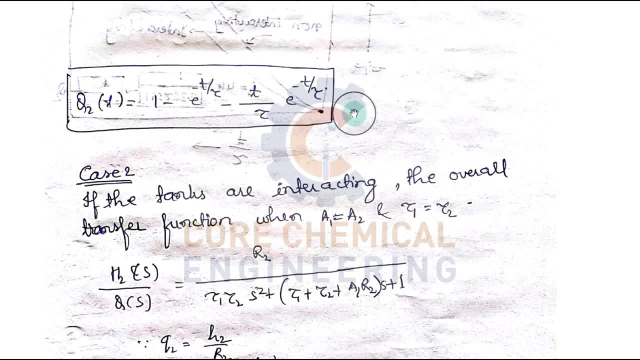 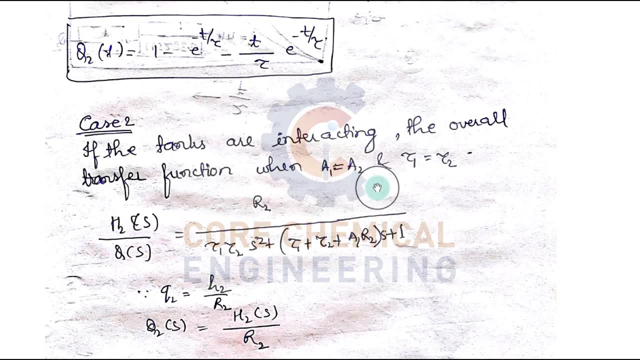 So this is very important. You must practice this also For case 2, if the times are interacting and the overall transfer function, 1, a1 is equal to a2 and tau 1 is equal to tau 2.. a1 is equal to a2 and tau 1 is equal to tau 2.. 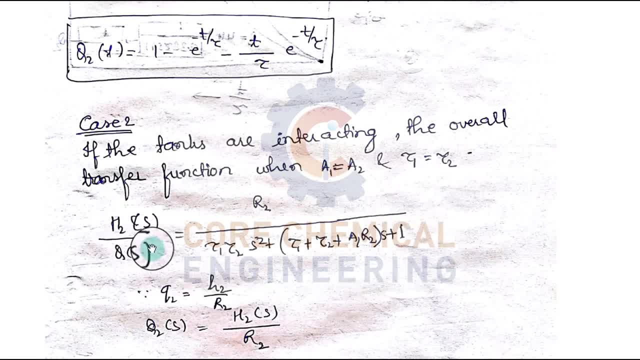 So we know that for non-interacting system, h2s divided by Q of s is equal to r2 divided by tau 1 into tau 2 into s square plus in bracket tau 1 plus tau 2 plus a1 into r2. in bracket close s plus 1, okay. 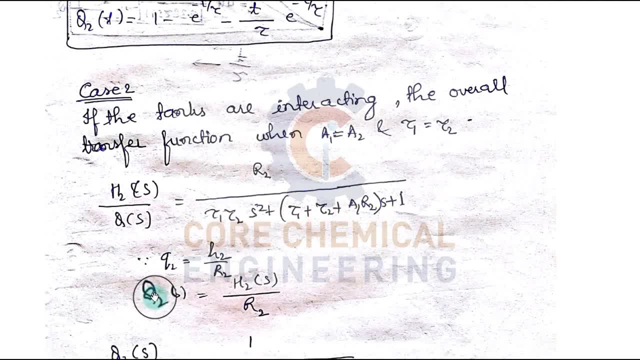 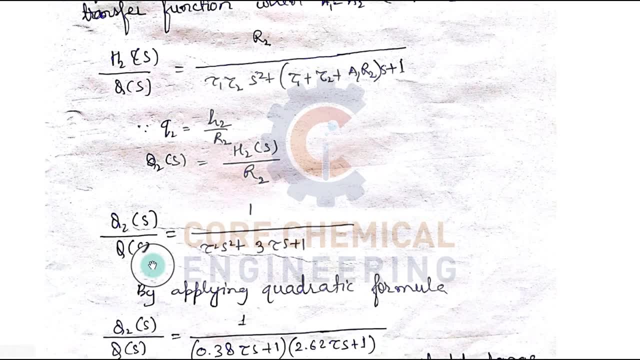 So what we need to do? We need to do this. Just put: Q2 is equal to h2 by r2.. We know now Q2 of s is equal to h2 s divided by r2.. So we will get: the value of Q2 s divided by Q of s is equal to 1 divided by tau, square, square plus 3, tau s plus 1.. 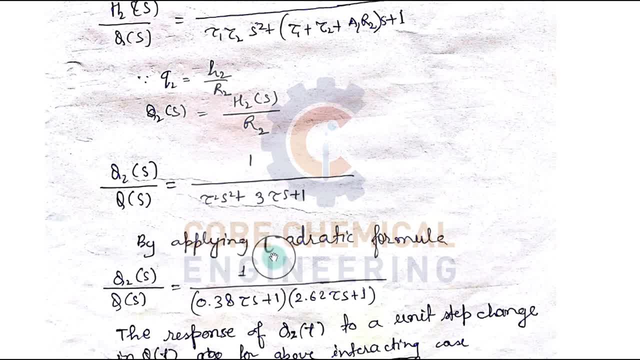 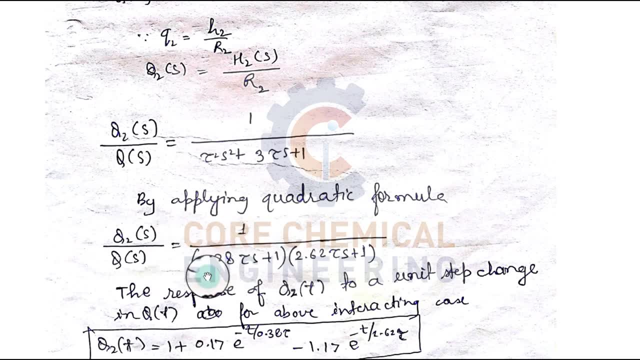 So we can solve this equation by using the quadratic formula. So if you solve it by using the quadratic equation formula, we will get Q2 s divided by Q of s is equal to 1 divided by 0.38 tau s plus 1 in bracket. close. 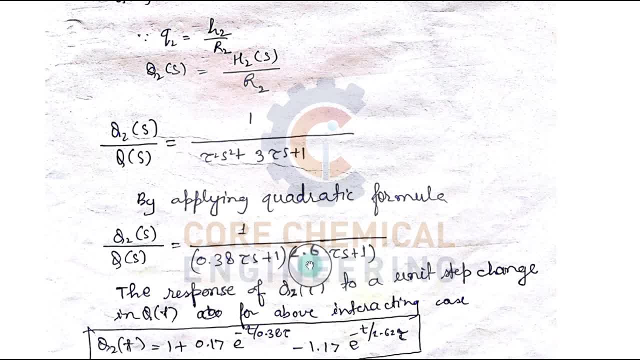 Now in bracket 2, point 2, point 6: 2 tau s plus 1, okay, So this is what we will get, that transfer function for non-interacting system when a1 is equal to a2 and tau 1 is equal to tau 2, right. 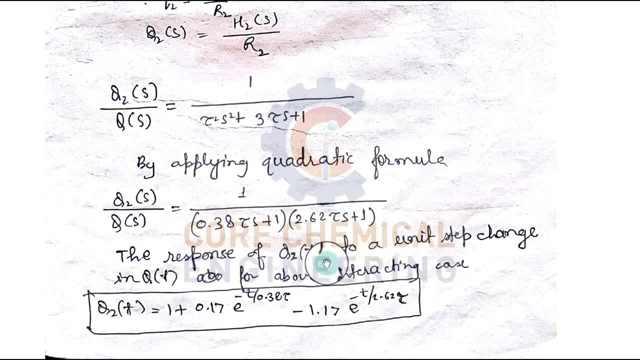 Now the response of the Q2 of t to a unit step response in Q of t for above interacting system. So if we are going to give the unit step input, means Q of s is equal to 1 by s. okay, 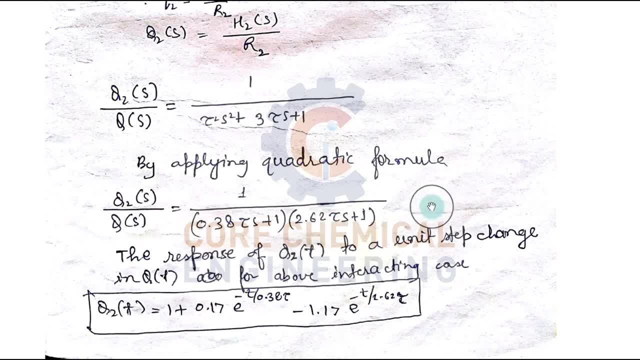 In that condition, if we solve this value, solve this equation and want to calculate Q2, Q2 of t means outlet flow rate. okay, In that in that case is equal to 1 plus 0.17 e raised to the power minus t divided by 0.38 tau minus 1.17. 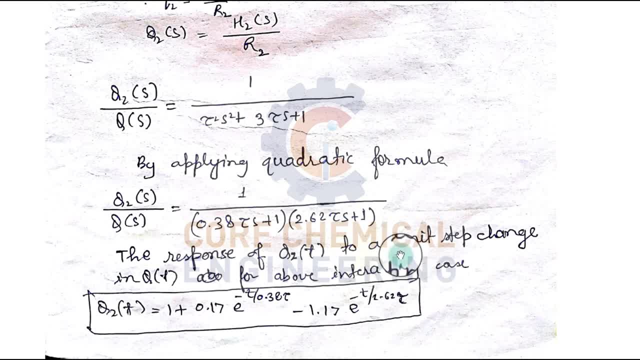 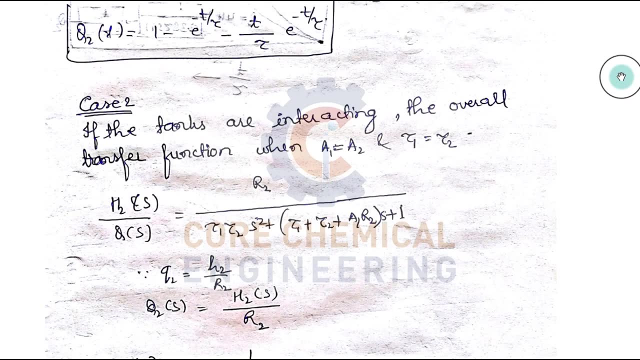 into e raised to the power minus t divided by 2.62 tau. So that's all for interacting system. Hope you guys understood it. understood it well, and guys, I had as of now covered five to six tutorials and the link of all those tutorials from the subject and I sight control. 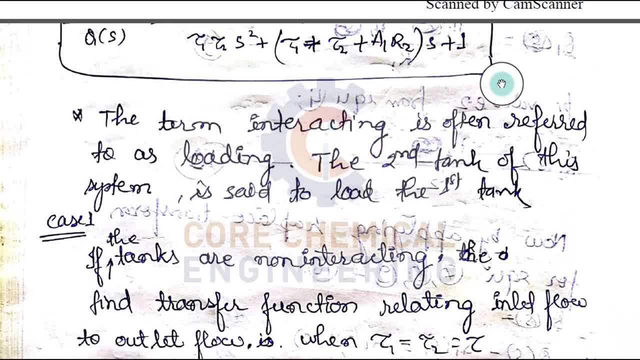 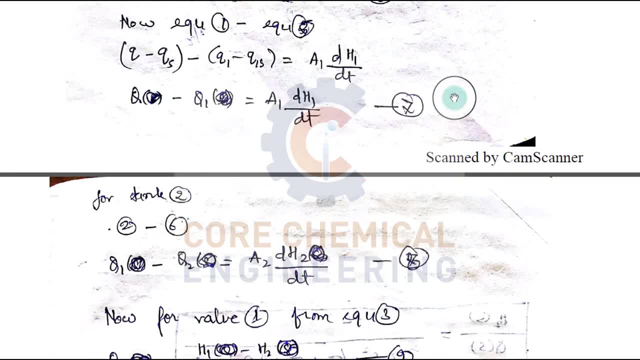 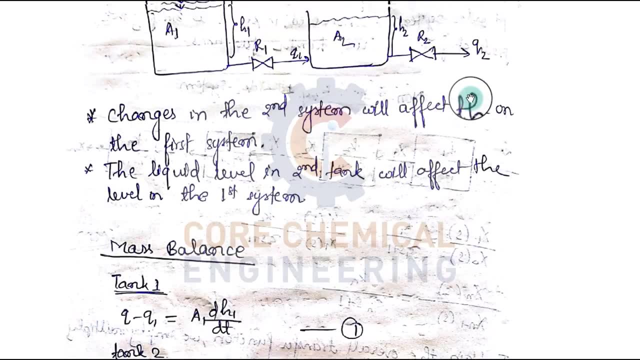 Okay, I'll give the link in the description box. if you want to refer those tutorials, you guys go and click on those links and Watch those videos. So that's all, Thank you. Thank you so much, And one more request is there from you guys: if you do like this video, please share among your friends, colleagues and Junior and 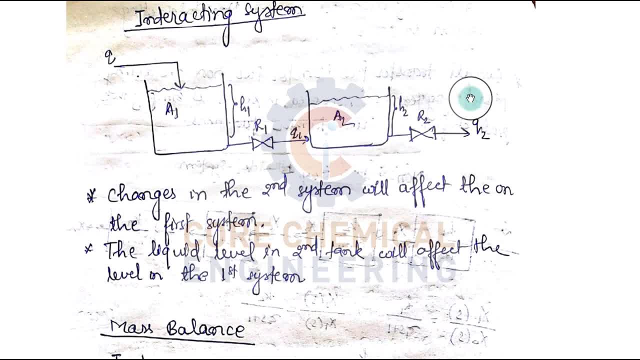 and if you want to know anything else apart from this video, you can comment into the comment box. I'll definitely reply in the form of comment or I'll make the video publish the tutorial. so that's all. and one more request is there again from you guys that if till now, if you haven't subscribed this channel. 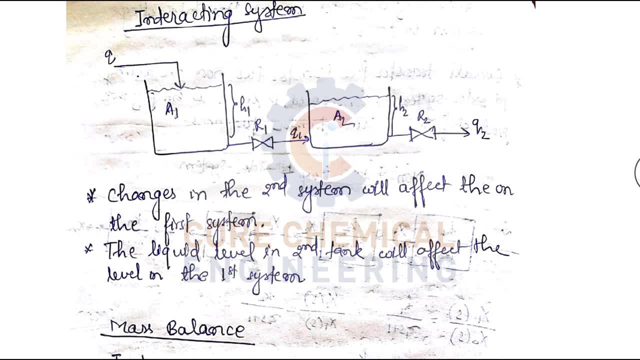 please do subscribe this channel and share as much as possible. thank you, thank you so much.